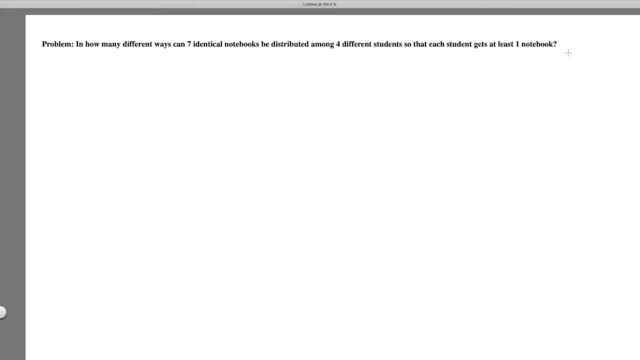 Okay, let's see how we do this. So in how many different ways can seven identical notebooks be distributed among four different students? So one way of simplifying this question is, instead of consider four different students, let's consider fewer students. So let's look at first. 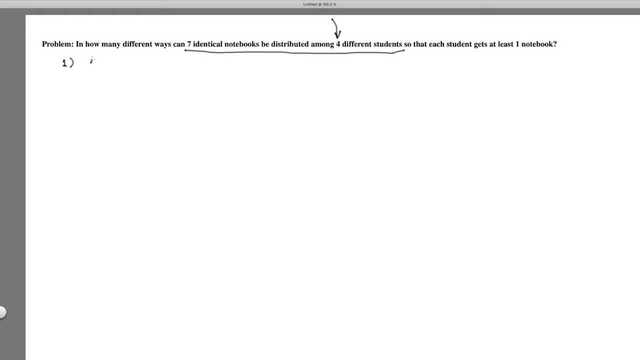 Instead of four. let's consider there's only one student, And the question becomes: in how many different ways can seven identical notebooks be distributed among one student so that each student gets at least one notebook? All right, that, of course, is a really obvious problem. 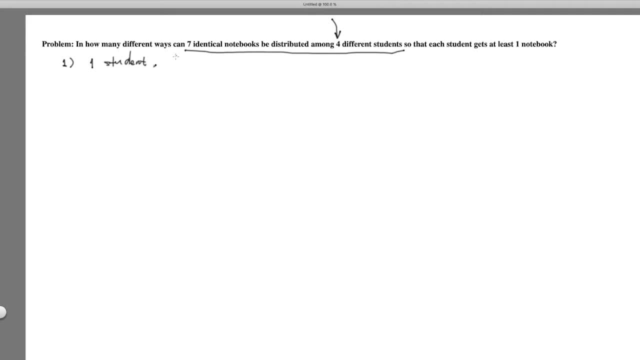 It's very simple, In fact: instead of seven identical books, let's consider n identical books, And n is bigger than or equal to one, And clearly there's only one way: You just give all the books to that one student. 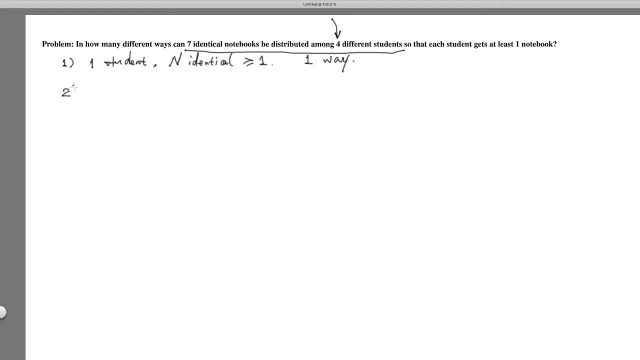 All right, so this is a trivial case. Now, instead of one student, let's consider there are two students And again there are n books. How many different ways Now we use casework. For the first student if you get one book. 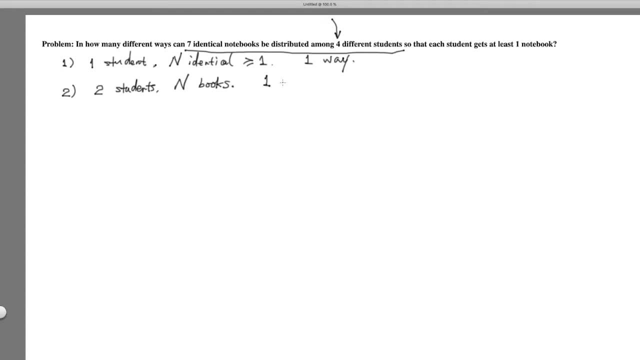 then all the n minus one books go into the second student. If you get two books for the first student, then all the n minus two books go into the second student. So clearly and so on. so clearly, the first student if the first student gets one or two. 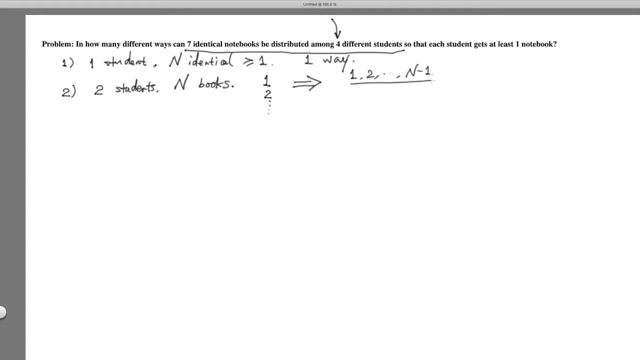 or n minus one books, each way corresponding a different way of distributing those books to among the two students. So totally, there are n minus one ways. Remember this. n minus one ways is basically I have n books And two students. 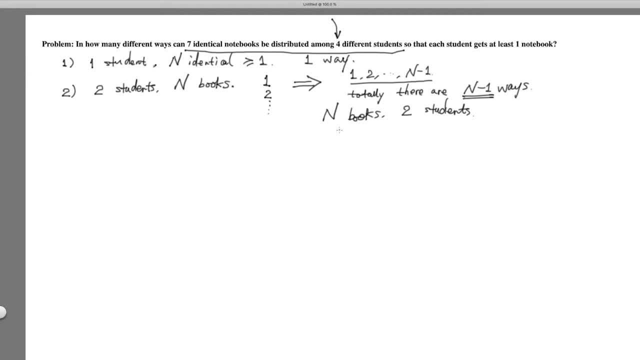 And again, this question is pretty simple, right? If you just look at this question at the first, how many ways I distributed n books to two students? it's very easy to arrive at this solution: n minus one ways, because the first student can get either one, two or three. 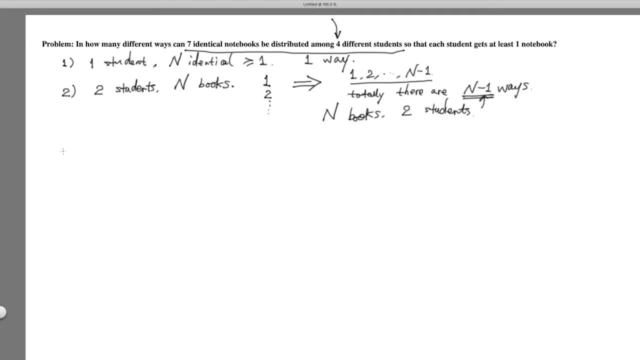 And then afterwards it's just determined. Okay, Now the third case is slightly more complicated. Let's say there are three students and n books. The idea is, again, we're going to consider the casework for the first student. 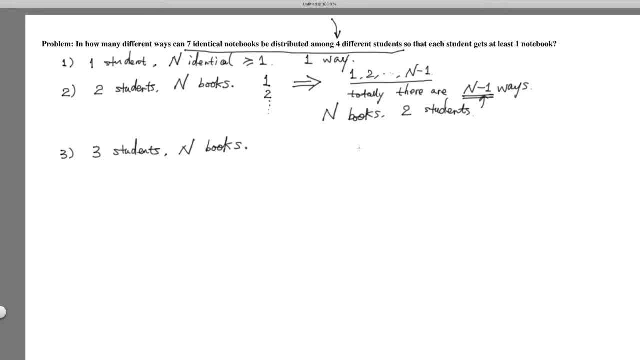 and then we're going to use the result that we already got of the number of ways disputing n books to two students, Because once you get, once you distribute the number of books to the first student, the remaining problem becomes distributing the remaining books. 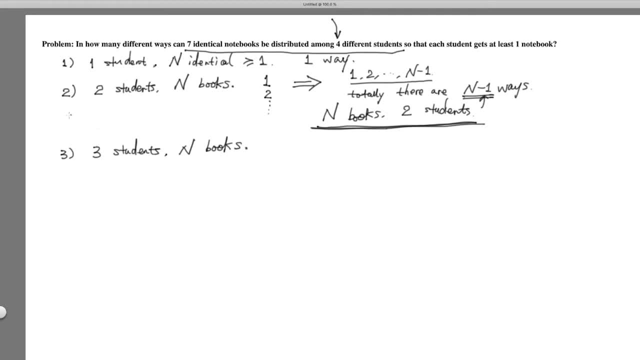 to the other two students, Right, And that will be a problem for the second case. Let's see If the first student, if the first student, gets one book. so the problem now becomes: we need to distribute now n minus one books. 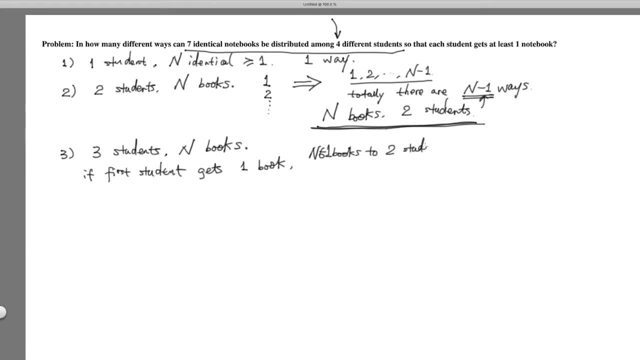 to two students. By the result we already got from case two, if n books given to two students there are n minus one ways, then for n minus one books to two students we have n minus two ways If first student gets two books. 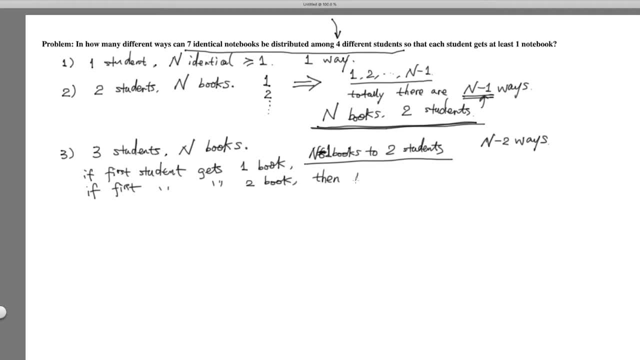 then we're going to distribute n minus books- because that's the remaining number of books- to the other two students, And this again by using the result. in the case two, we have n minus three ways. And similarly, if the student gets, 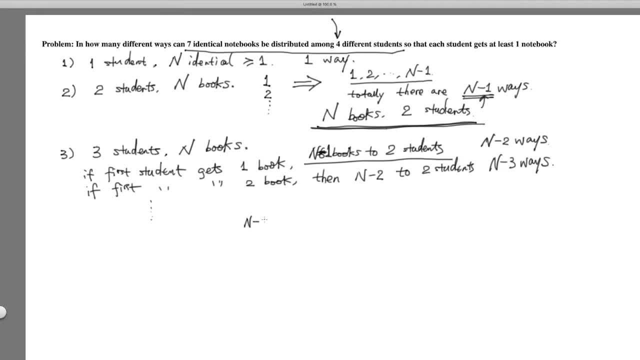 n minus two books, then the remaining two books to the other two students. There's only one way. Notice that there's this pattern going on. If there's n minus two books, there are n minus three ways for giving to two students. 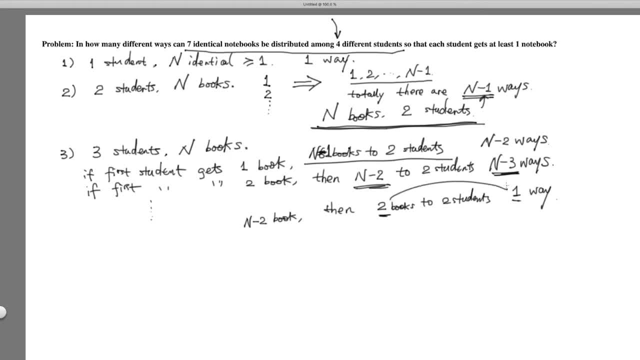 If there are two books, there are one way, So the difference always is one. Right? That's the way you're kind of checking your answer. All right, So that means, if I sum up all those different ways, that's exactly the total number of ways for. 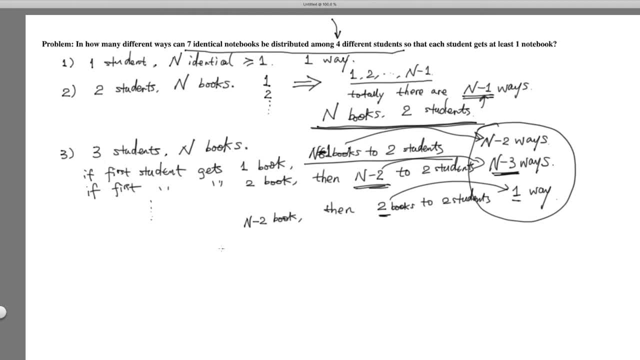 distributing n books to three students, And the result of that would be n minus two plus n minus three plus all the way to one, And that, of course, using the summation formula for one plus two plus all the way to a positive integer. 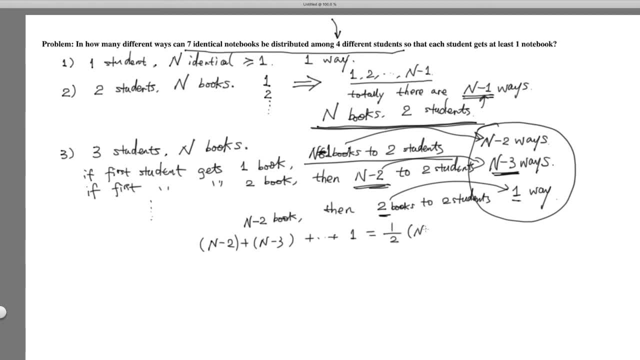 that equals half of n minus two times n minus one And again. doing this sum is: remember that you just can reverse the total numbers and then you pair them together. This formula, All right, Remind yourself what this formula is. This formula says that: 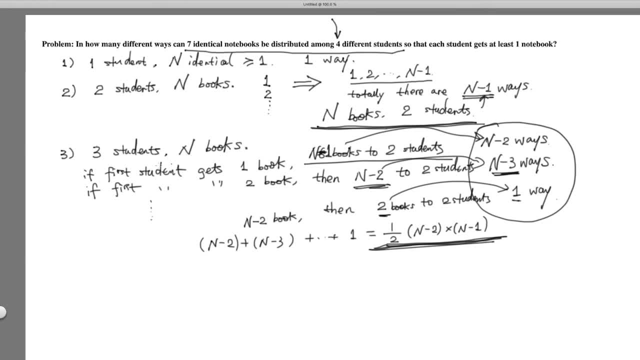 this is the number of ways of distributing n books to three students. So we have done this case. Now let's come to the final case that we want to solve the problem at hand for four students and seven books. Of course we can actually. 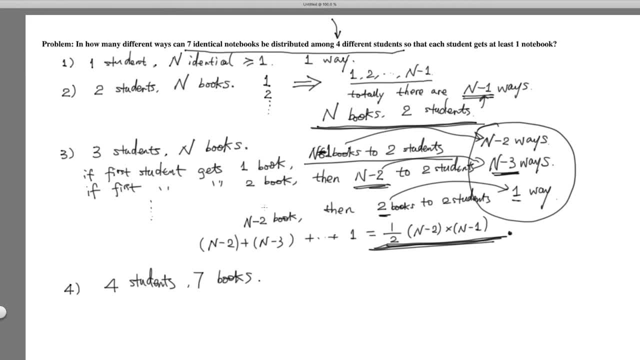 solve it for any n books, but this problem is only for seven identical books. So let's do four students, seven books. Again, we're going to do the casework of how many books the first student gets and then, using the result, 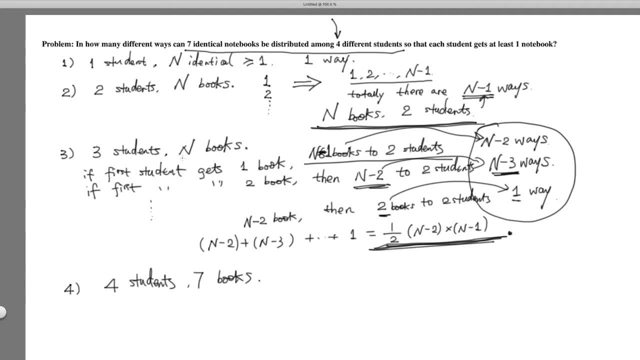 we already got for three students of arbitrary n books. we have this formula using that result for the casework: All right, Case number one If the first student gets one book. So the total number of ways for this case is going to distribute. 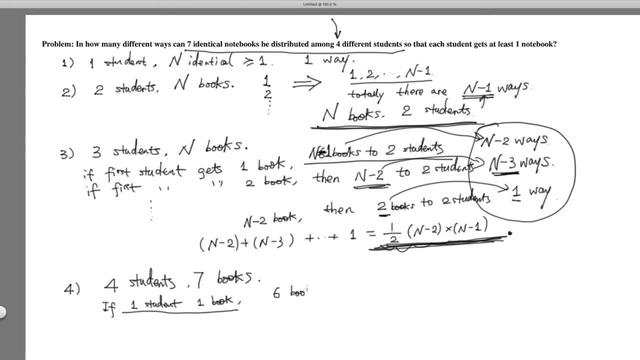 the remaining six books to the other three students. And because of case three, we know that this is the total number of ways. okay, for n equals six, So this total number of ways is going to equal half times six minus two, six minus one. 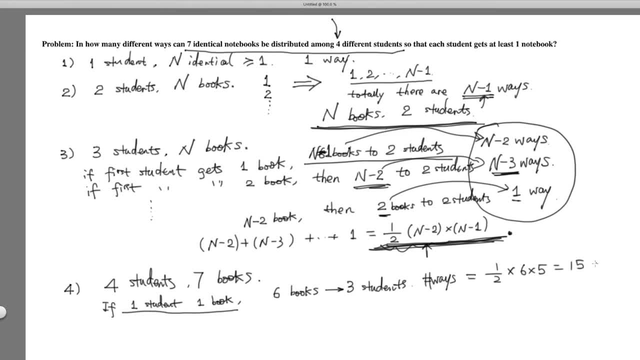 six times five equal 15 ways. Sorry, n equals six, so four times five equal 10 ways. If the first student gets two books, in this case we're going to distribute the remaining five books to the other three students. 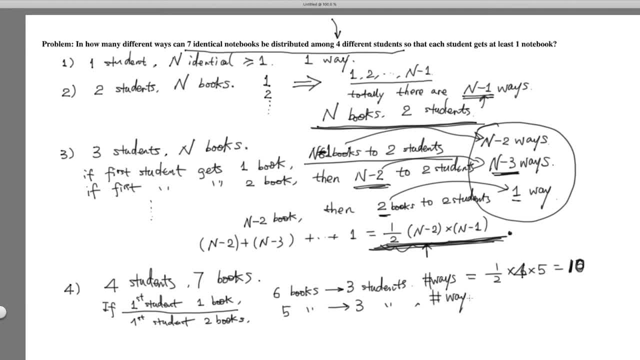 And the number of ways is again using this formula: Distribute n books to three students. is this formula, So distribute the five books into three students is going to be half of three times four. six ways: First student get three books, So that will be four books. 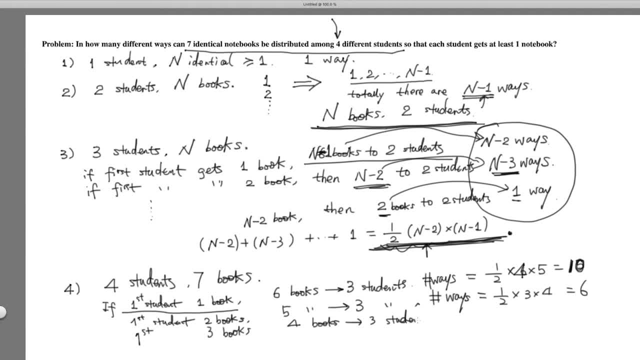 go to three students. Number of ways equals half times two times three equals three ways. And finally, if the first student gets four books, then the remaining three books goes to three students And clearly there's only one way, because each one gets one book. 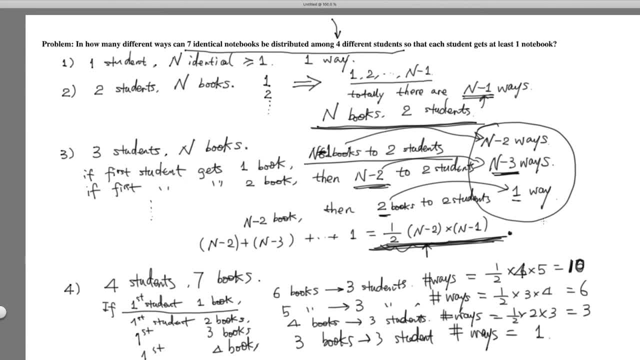 So the total number of different ways is going to be, adding all those things together, 10 plus six plus three plus one. Total number of ways is 10 plus six plus three plus one equals 20.. Okay, let's review a little bit.